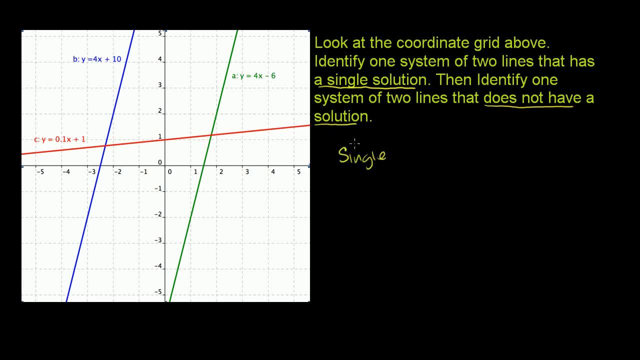 So a single solution And they say: identify one system. but we can see here, actually there's actually going to be two systems that have a single solution, And when we talk about a single solution, we're talking about a single x and y value that will satisfy both. 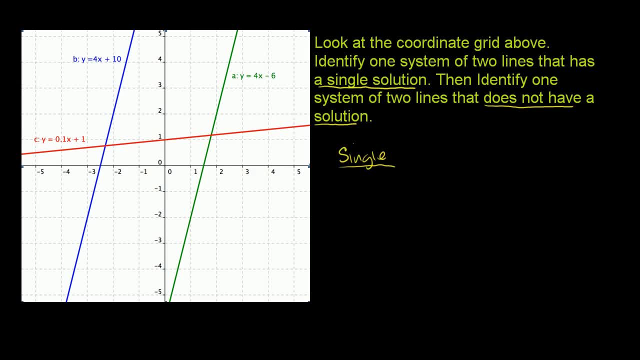 equations in the system. So if we look right here at the points of intersection, this point right there that satisfies this equation, y is equal to 0.1x plus 1.. And it also satisfies this blue line. but the graph that 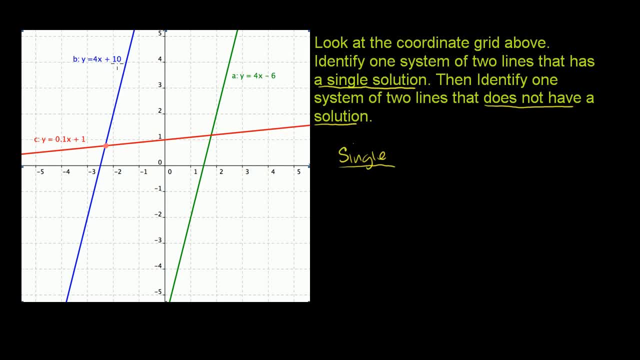 that line represents y is equal to 4x plus 10.. So this dot right here, That point, represents the solution to both of these, or, I guess, another way to think about it, it represents an x and y value that satisfy both of these constraints. 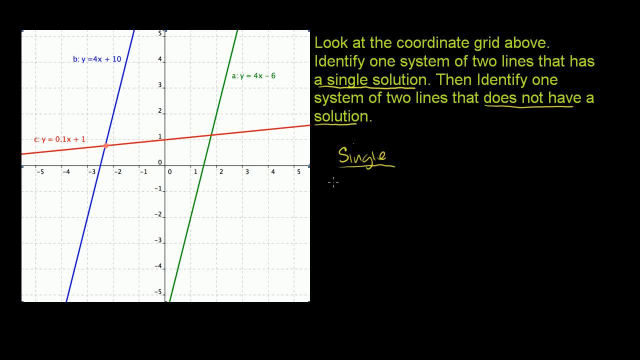 So one system that has one solution is a system that has: y is equal to 0.1x plus 1.. And then this blue line right here, which is y is equal to 4x plus 10.. Now they only want us to identify one system of two. 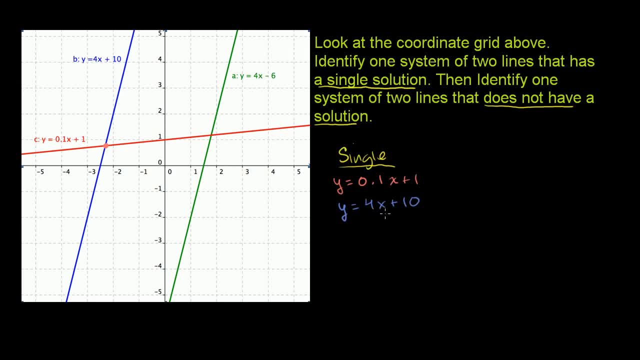 lines. that has a single solution. We've already done that, but just so you see it, there's actually another system here. So this is one system right here. or another system would be the green line and this red line, This point of intersection right here. once again, that. 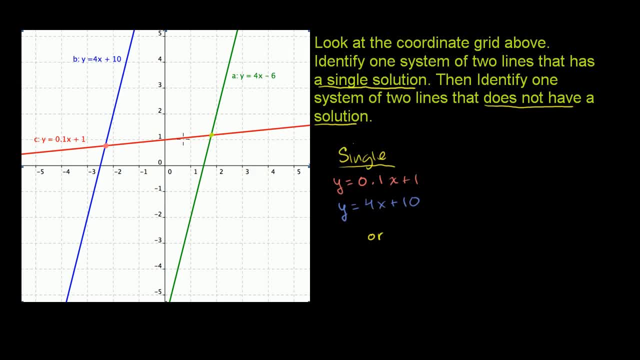 represents an x and y value that satisfies both. the equation y is equal to 0.1x plus 1.. So y is equal to 0.1x plus 1.. And this point right here satisfies. the equation y is equal to 4x minus 6.. 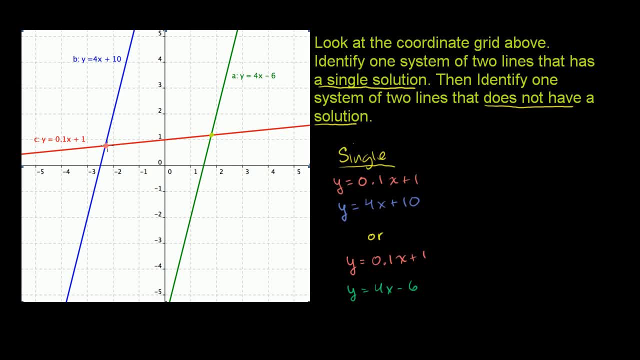 So if you look at this system, there's one solution because there's one point of intersection of these two equations or these two lines, And this system also has one solution because it has one point of intersection. Now the second part of this problem. they say: identify one.